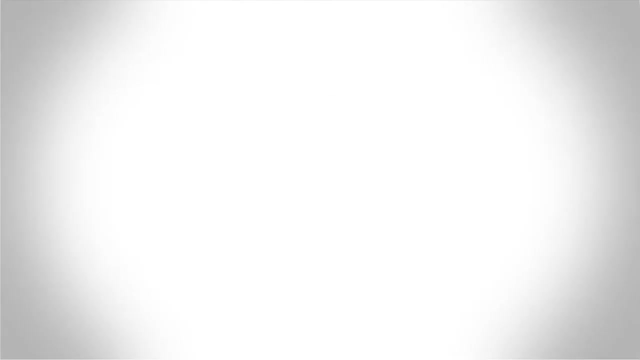 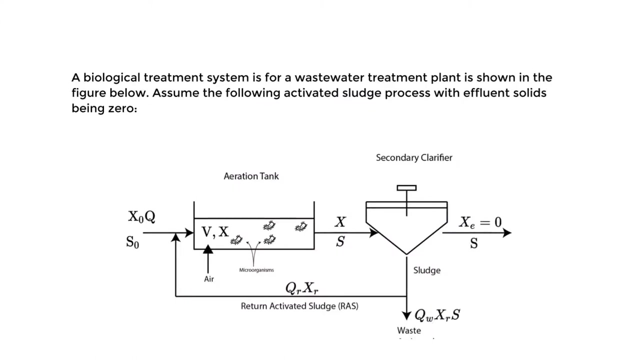 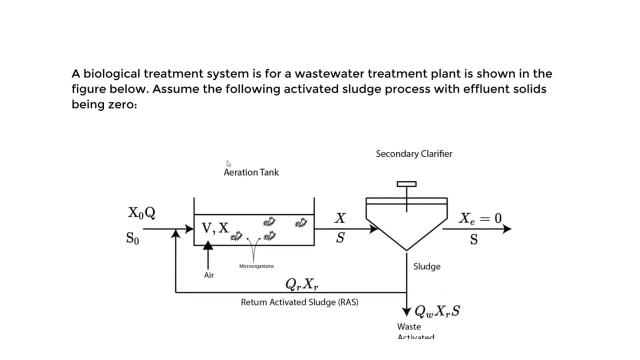 Okay. so now let's look at the activated sludge process and determine the return recycle flow rate. that is going to be, specifically, our Q sub R. So here we have a biological treatment system, is for a wastewater treatment plant and is shown in the figure below. We're going 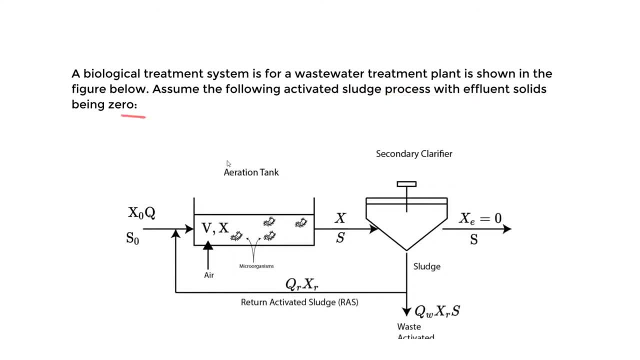 to assume the following: activated sludge process with effluent solids being zero. So this is key here: the effluent solids here are going to be zero. This is what we're assuming. This is our X sub E, This will be our effluent solids and we're going to say, at the effluent, 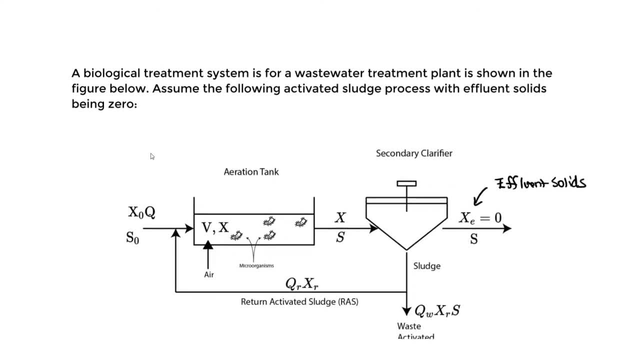 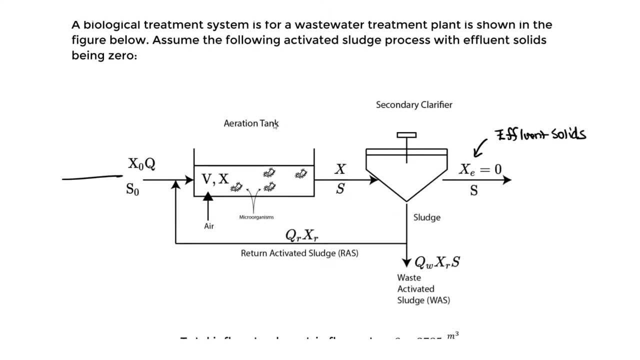 when we exit, it's zero. So we know, here we have a activated sludge process, we have a aeration tank and a secondary clarifier. So this is where we enter, This is the inlet, This is the effluent, This is where we exit. 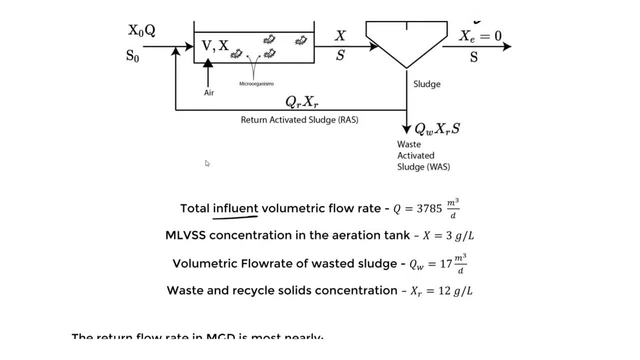 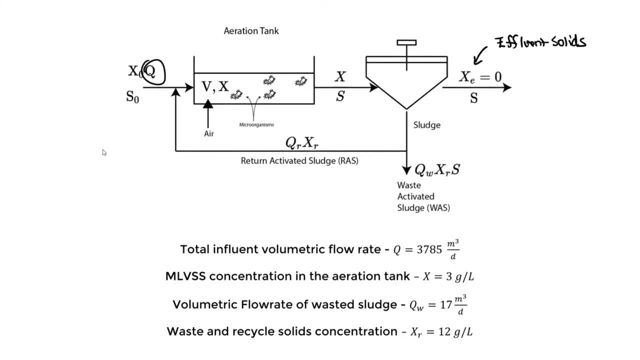 And we know here that we're given the total influent volumetric flow rate. So this is the total flow rate and it's going to be our Q. It's just this Q. We know the MLVSS, the mixed liquor volatile suspended solid concentration in the aeration tank, is 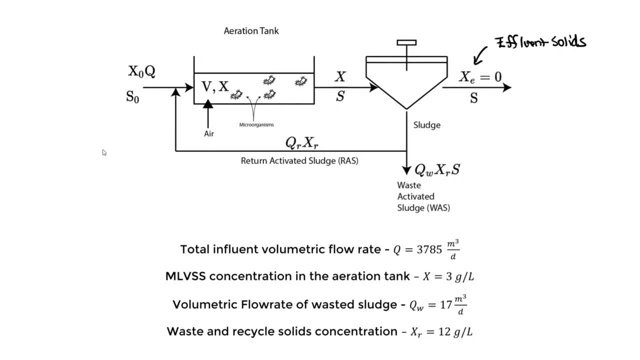 X. So this is going to be this value And this is for the aeration tank which has the microorganisms And we know, since we have X here, this is what's going to exit our aeration tank And this is given to be 3 grams per liter. 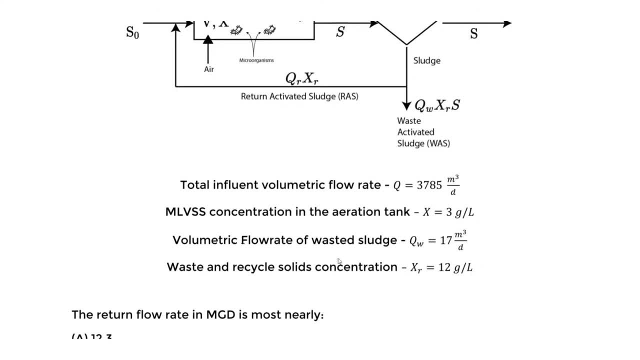 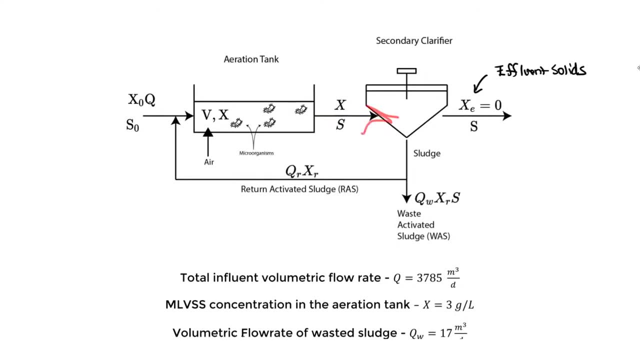 Then we have the volumetric flow rate of the wasted sludge is given to be Q sub W. And where is that? We know that we enter at some flow rate, at some X and some S. And a side note here: We know X relates to the cells. 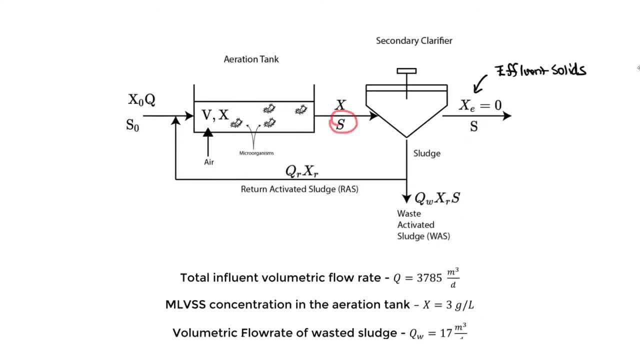 S is the sewage. So this is the sewage At the effluent. it's the same as the sewage entering the secondary clarifier And we know this is the sewage initially at the influent, the initial sewage we're looking to treat. 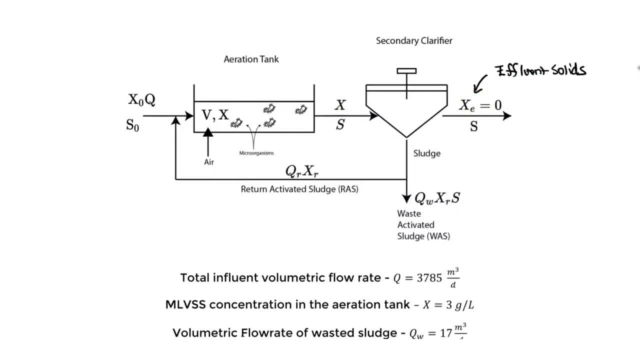 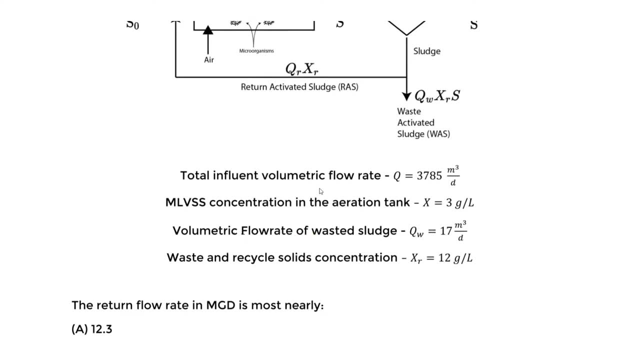 S stands for sewage X. you can think of it as here, effluent solids. It relates to the cells. So we know here that Q sub W is the volumetric flow rate of the wasted sludge, And it's going to be this: 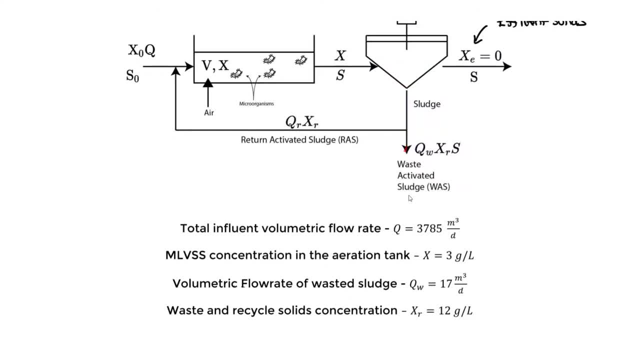 So here, from the secondary clarifier, We have some sludge. Part of it is going to be get returned- And this is what we call the return activated sludge- And part of it is going to be wasted, And the wasted is going to be Q sub W And it's going to be the waste activated sludge. 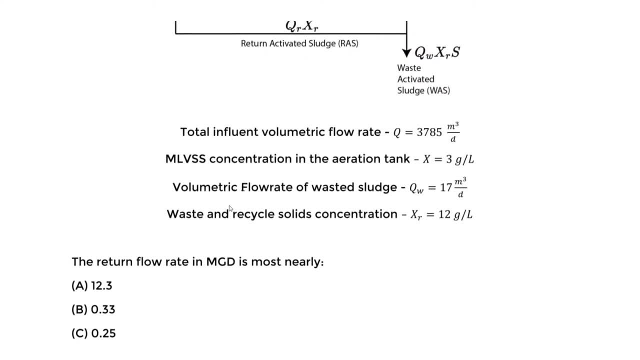 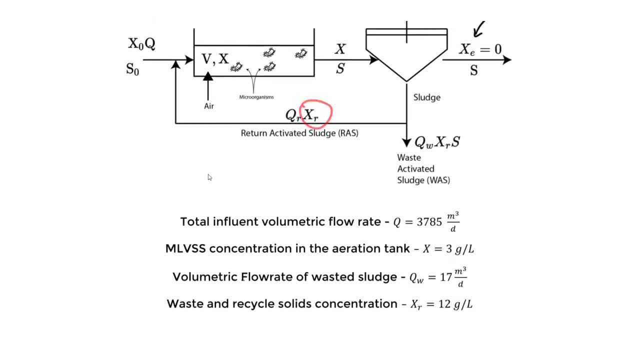 which has a flow rate Q sub W. So we're given that And we're told the waste and recycle solids concentration Q sub R is given. So Q sub R here for the return, activated sludge is given to be 12 grams per liter. 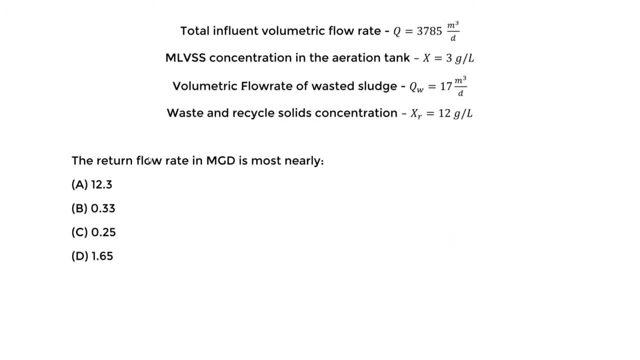 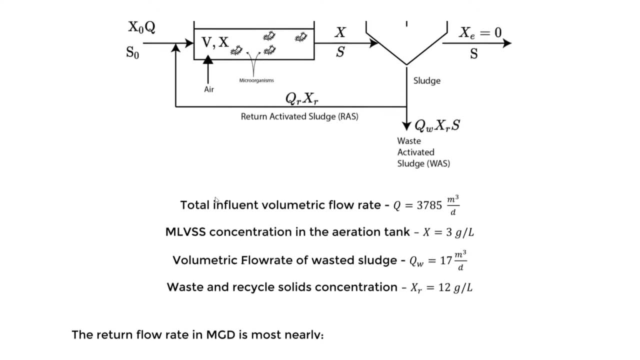 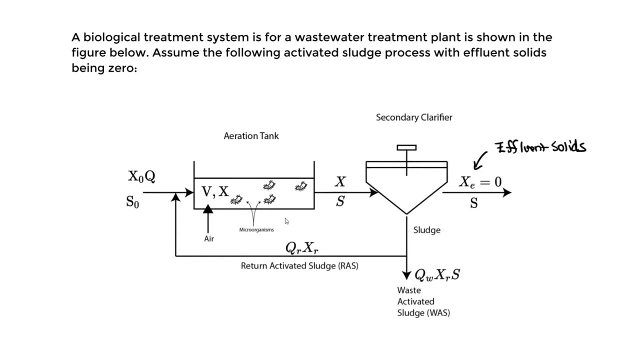 So what do we want to find? We want to find the return flow rate in million gallons per day. What is this monsoon area? So how do we do this? What I propose here is to do a mass balance. But which system do we want to isolate for a mass balance? 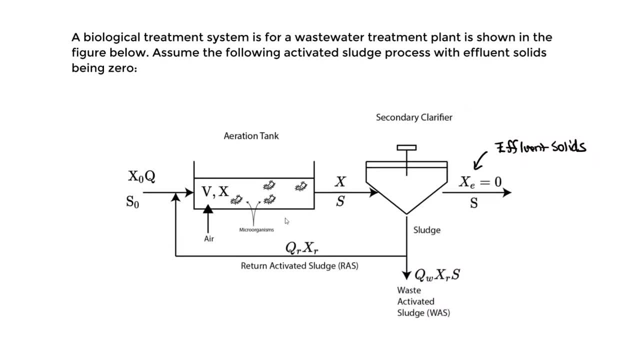 We can do the overall system, But I notice that we're looking at this return activated sludge And that is mainly concerned with the secondary clarifier. So what we're going to do is isolate the secondary clarifier And I'll just make a box around it. 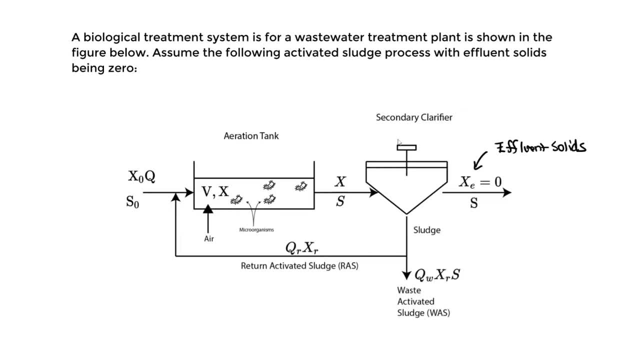 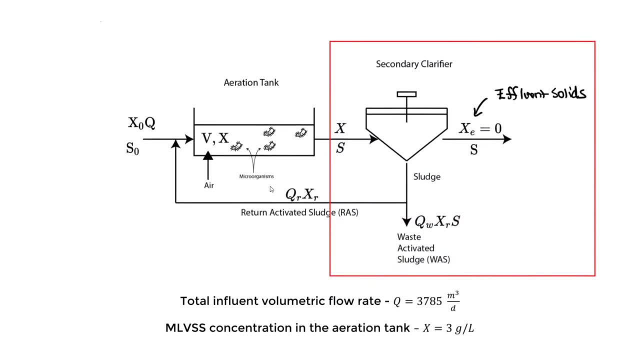 Being that we know we're going to analyze strictly just the secondary clarifier And we're going to apply a mass balance to it, With the end goal of finding Q sub R: The flow rate, the recycle flow rate which relates to the return activated sludge. 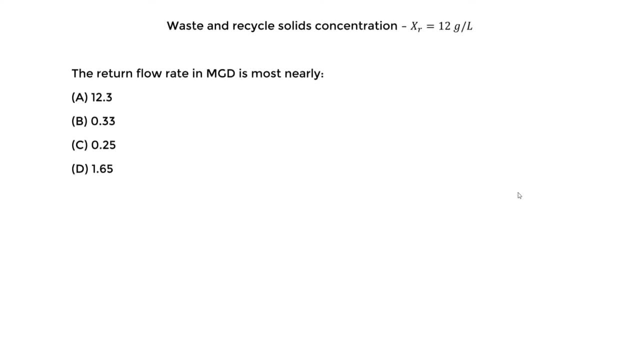 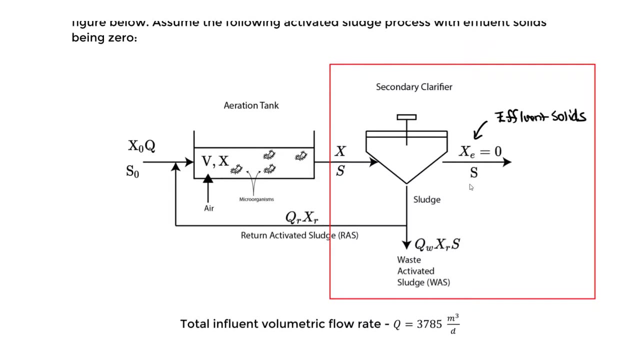 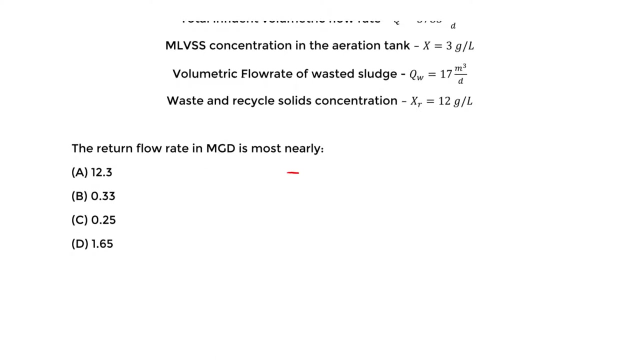 Right. So here, first thing is: we know we're isolating this and applying a mass balance. All that means is: whatever comes in has to equal whatever comes out. So what I'm going to say is, on the left side, Let's write: in equals out. 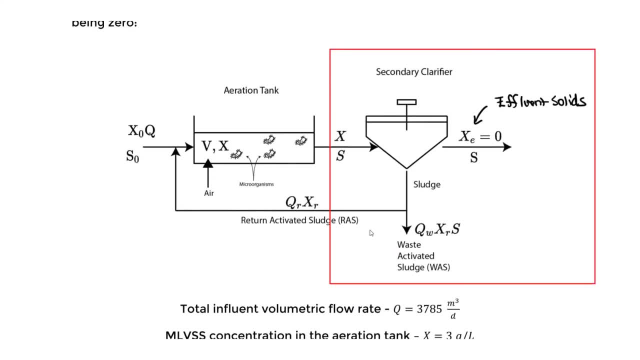 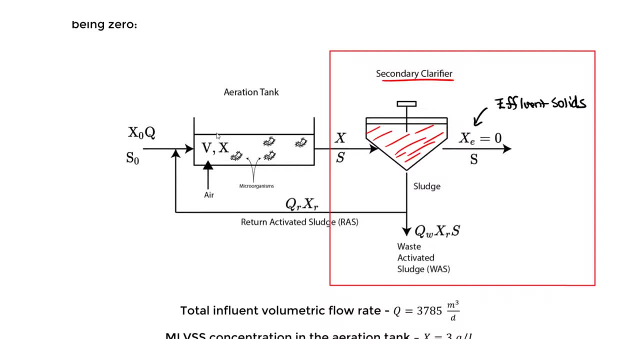 Okay. So we know let's look at what comes in Again, we're only looking at the secondary clarifier, So we're going to ask What enters our secondary clarifier, What comes in? So we know here that if you look, 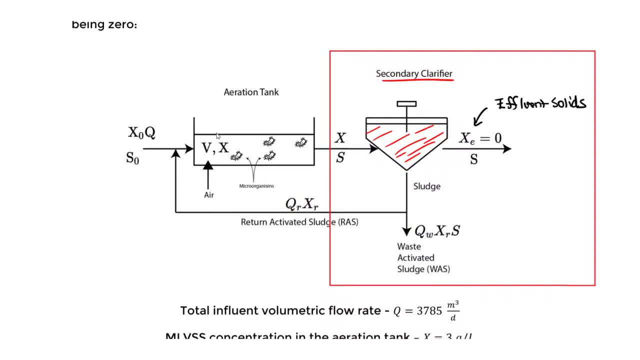 We have the sludge coming out down here, We have Q sub R that comes back And we have Q that comes in here. So we have a total of Q and Q sub R that enters at the influent, That enters the aeration tank. 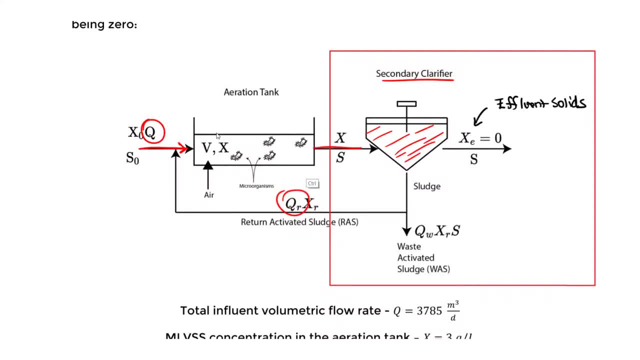 So whatever enters the aeration tank has to come out the aeration tank. So whatever comes in here Is going to be the total Q coming in here. So the total Q coming in here Will be our Q sub R plus Q. So it's going to be Q plus Q sub R. 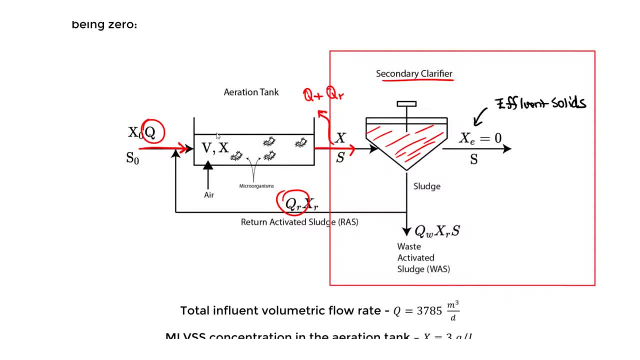 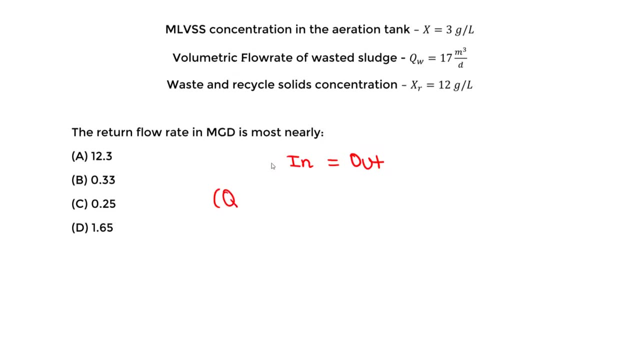 And here we take Q times our X value, Which is just that. So the total here is Q times X. So it's a mass flow rate. So we know, here On the end We have Q plus Q sub R, And we always multiply by the X value here. 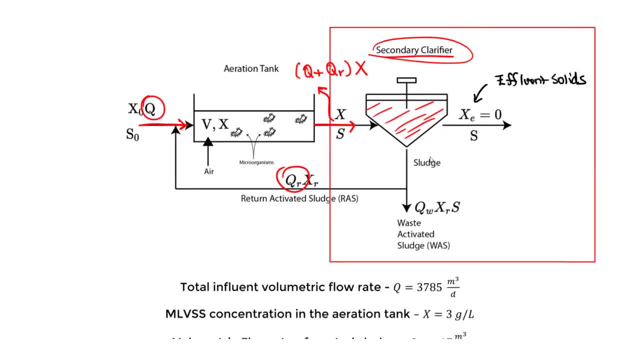 And that's what comes in here. Just strictly for the secondary clarifier, Once again, since this Q sub R comes back, It combines with the total flow rate that comes in here. So they combine together And that's why, whatever exit the aeration tank is going to be, 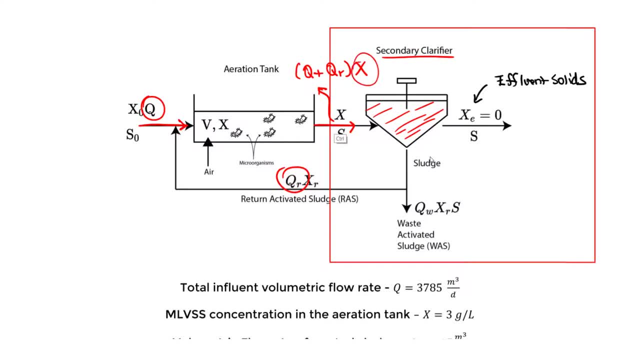 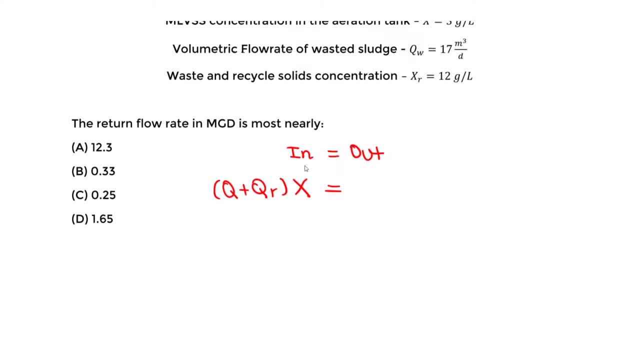 Q plus Q sub R, And all we did here is multiply by X This X value, and that is also given. It's the concentration. So that's going to be what comes in. That's all it is. So now let's look at what comes out. 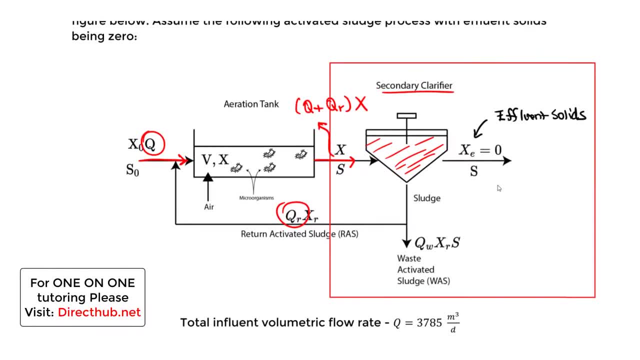 So let's look at the diagram, And the first one that we're going to look at, Which is going to be the easiest, It's going to be what comes out here. So we know that This Q Plus Q sub R. 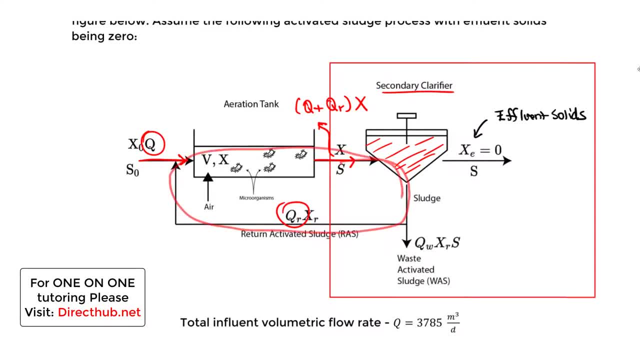 Comes in the secondary clarifier And it's going to be a cycle Just strictly for this. So in other words, We're only looking at Q plus Q R as a cycle, Just for this part Where we have the return activated sludge. 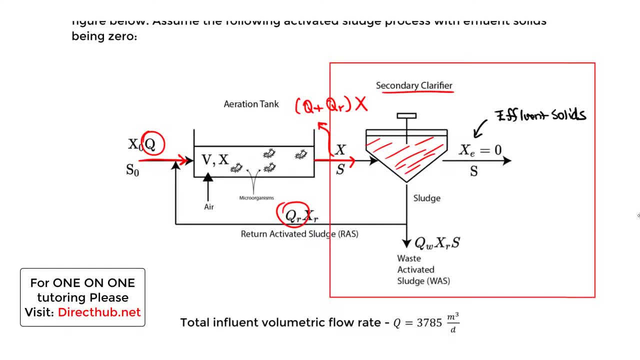 So here, whatever exits at the effluent, Essentially is going to be Q minus Q W. So we take the total flow rate coming in Minus the waste flow rate, Q sub W, And this is what's going to be at the effluent. 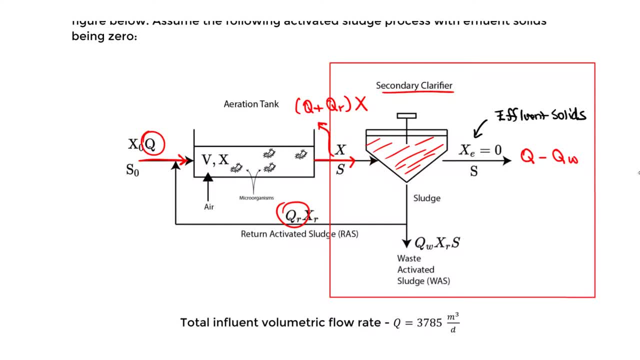 Because Q sub R Once again. We did not consider that. We know that comes in, But Q sub R is going to be. It gets recycled. That's our Q sub R, So it comes back around. But what exits here? 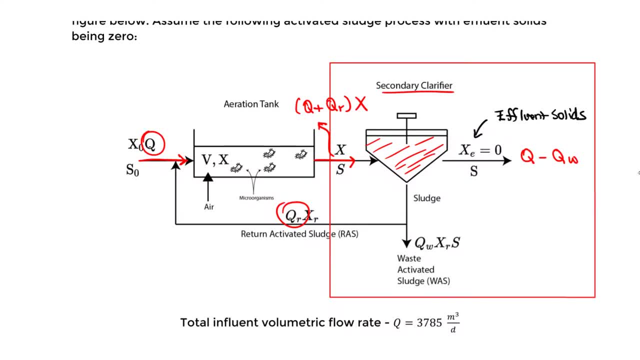 The effluent Depends on the total flow rate, Just the flow rate, The total flow rate Q, Not Q sub R. We do not consider that Minus what we waste, Q sub W. So that's going to be. 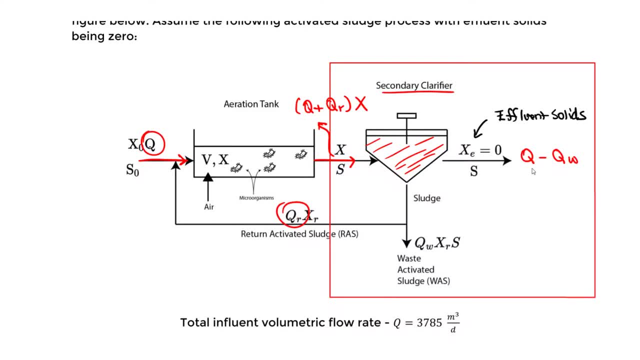 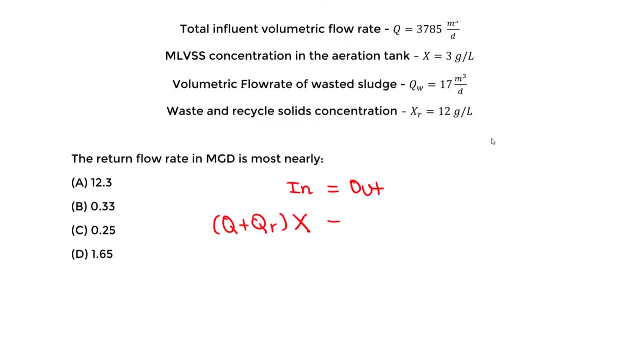 At the exit. So that's just An extra Note. But here, at the end of the day, We're not going to use this Because our X sub E is zero. So if I write it in my equation On the right side, 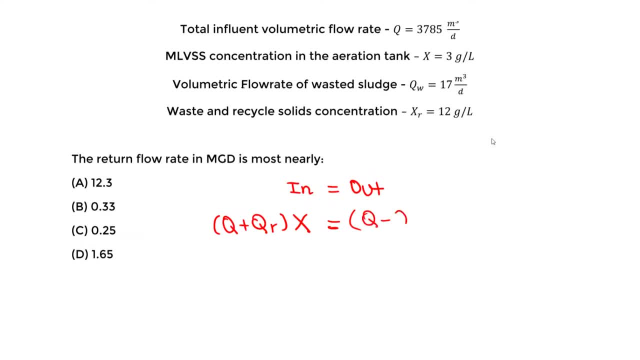 Whatever comes out here, We have Q Minus Q W. This is the flow rate at the effluent Times, X sub E. But we know X sub E is zero. So essentially this whole term goes away. So that whole term goes away. 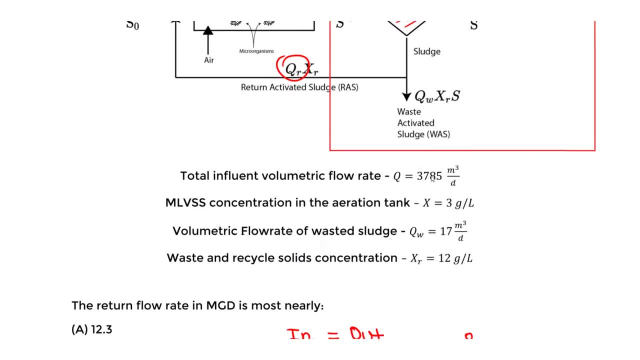 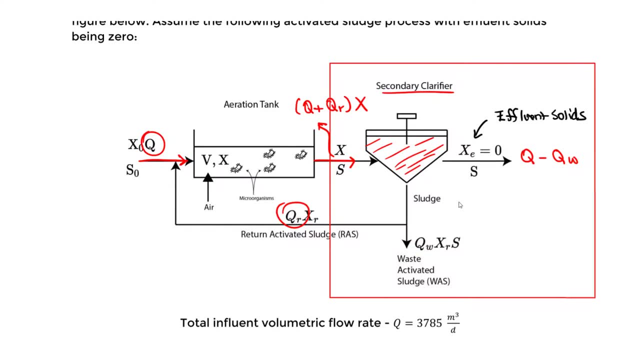 Because we're multiplying by zero. So we're not done yet. We have more things that come out, So we're looking at the secondary clarifier. What comes out here Is also going to be the waste activated sludge. So all you do is: 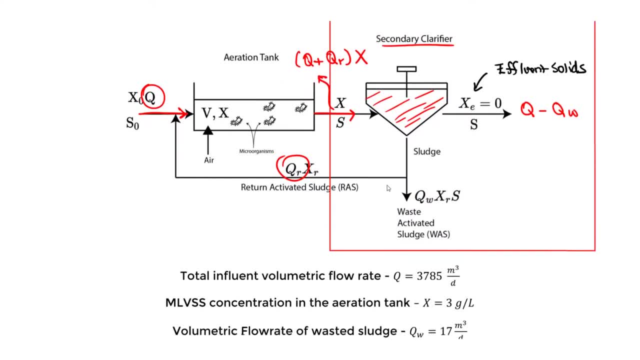 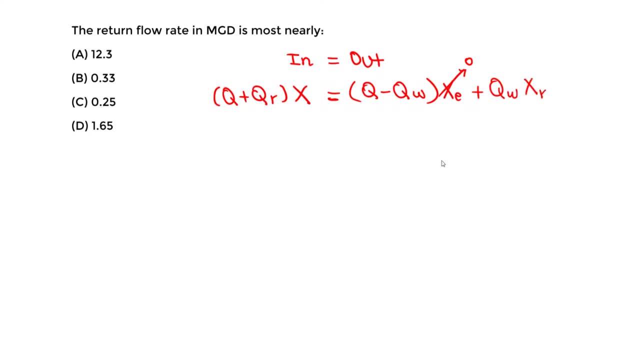 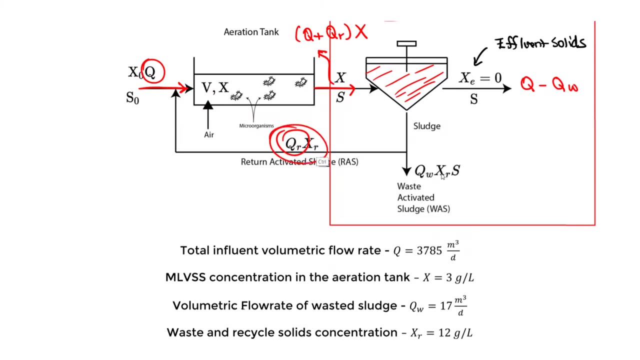 Q sub W Times X R. So we do Q sub W Times X R. Then we have Q R Times X R. So this also Comes out Right. Whatever comes out here Is this And this. So we have Q R. 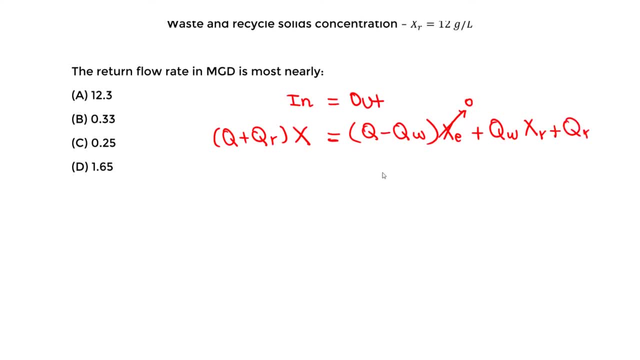 Times X, R. So now we're looking to solve for the return flow rate, Return flow rate, Which is going to be Q sub R. Let me highlight that So we know I can rewrite this equation By eliminating this Real quick. 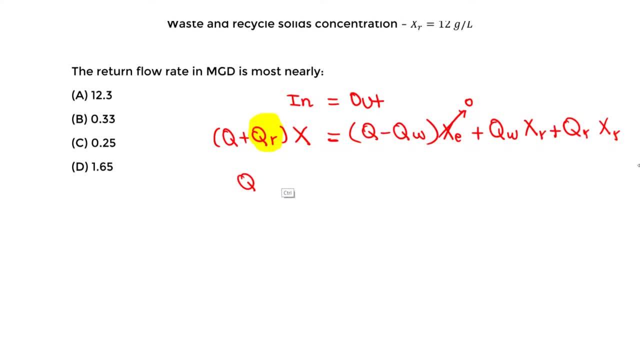 So we have Q plus Q R. Actually, what I'm going to do is Distribute the X. Let's distribute the X X times Q, So we have Q X Plus X times Q R. So it can be. 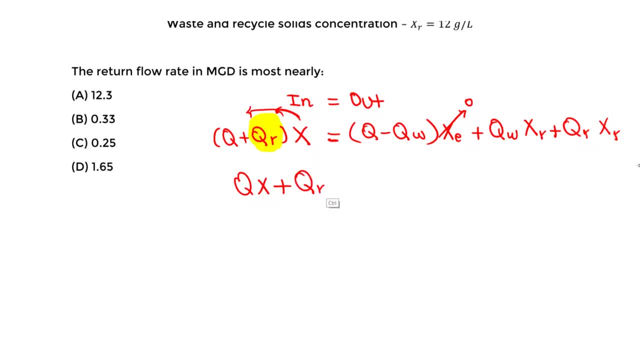 Q R Times X. So this is capital. X Equals to. So this whole term goes away, Because this is zero, We're told at the effluent, X Is zero, And so this is eliminated. So we have Q sub W. 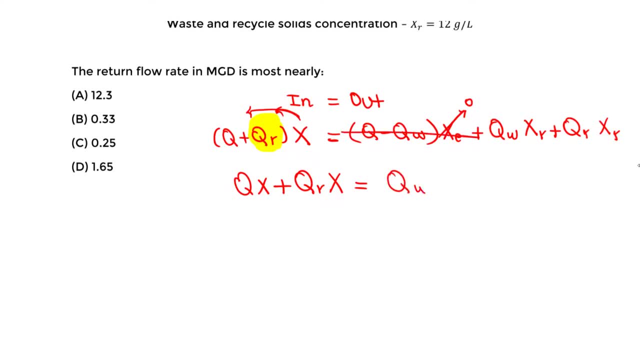 We have X sub R Plus Q sub R, X sub R. So now We're Looking at This Return flow rate. So now We're Looking to solve for Q sub R. Right, That's what we want to find. 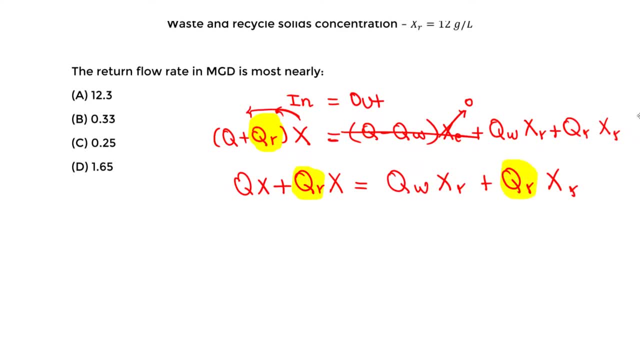 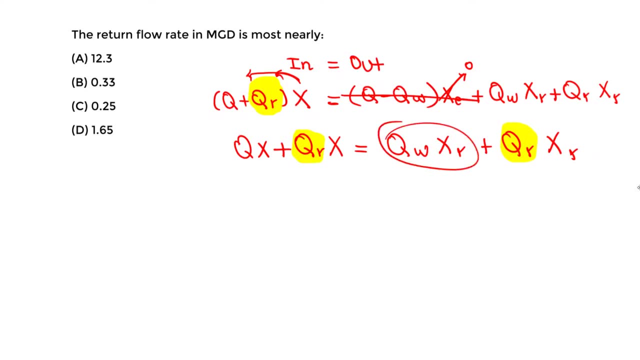 So It's Here And here. So I'm going to get those terms Next to each other. So we're going to rearrange The equation And I'm going to move This To this side And I'm going to move. 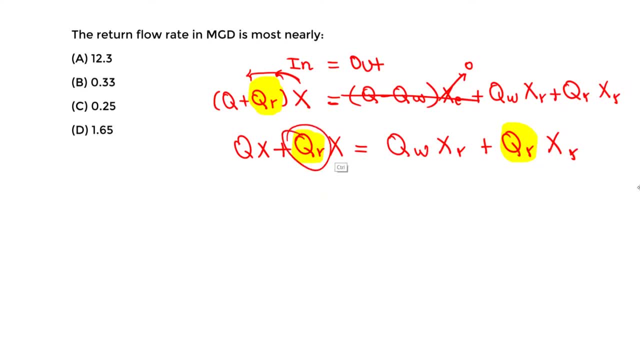 This To This side. I want these Next to each other, So We have Equals to. What you should get On the left side Is X Minus Q R. Times X R. 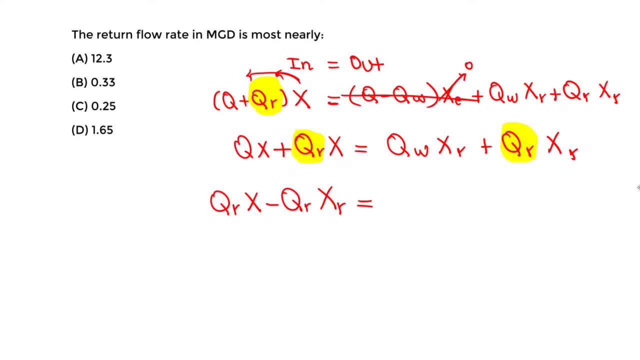 So all I did Was Move this To this side. Then I'm going to move This To this side. We're just doing Algebra Q R Minus Q Times X. So now We have. 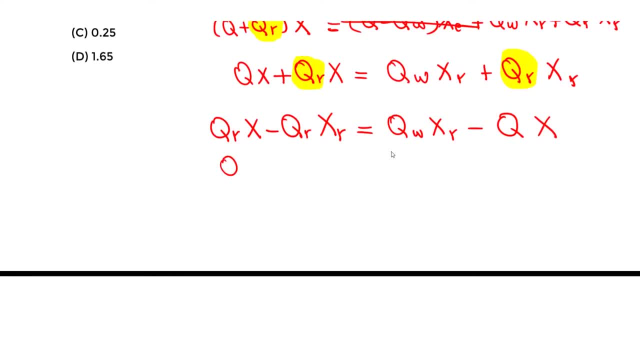 Q R On both sides, Which is Good. That's what we want: X Minus X R. I just took out A Q R Here Equals to Q W X R. 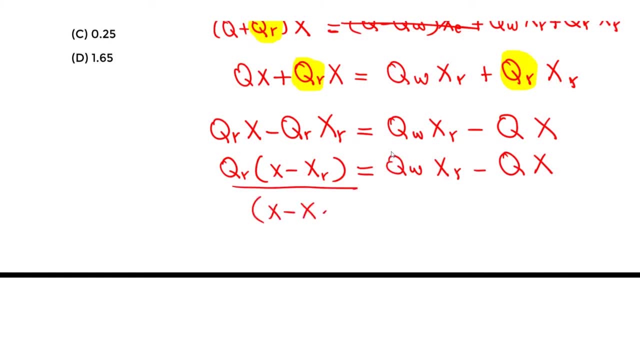 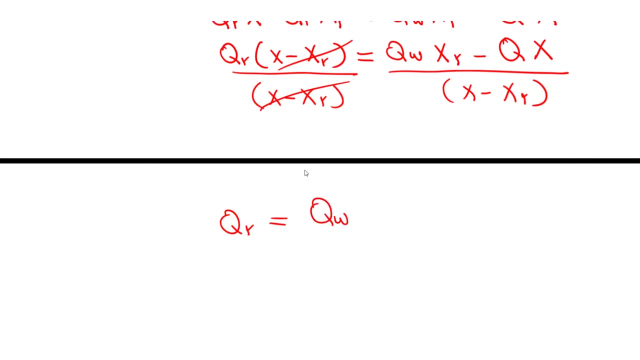 Minus Q Times X. So now We can solve For Q R You divide By X Minus X R And We know We're Given Q, W And